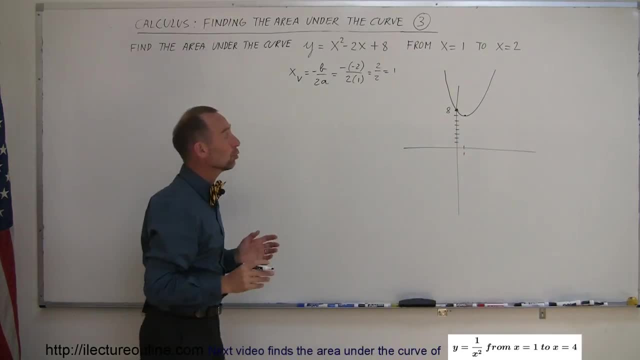 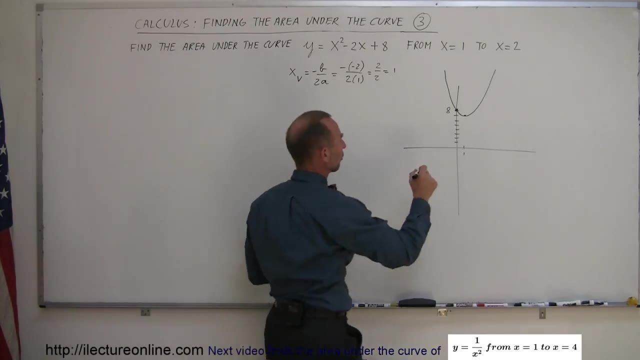 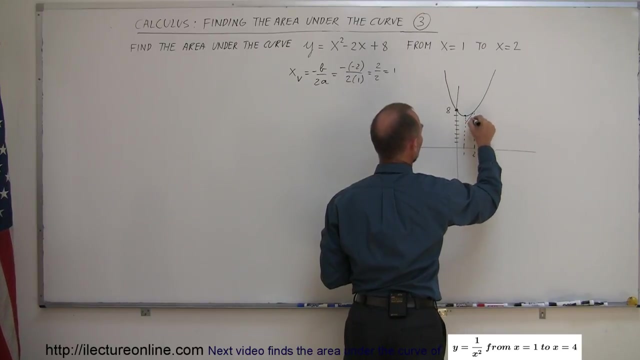 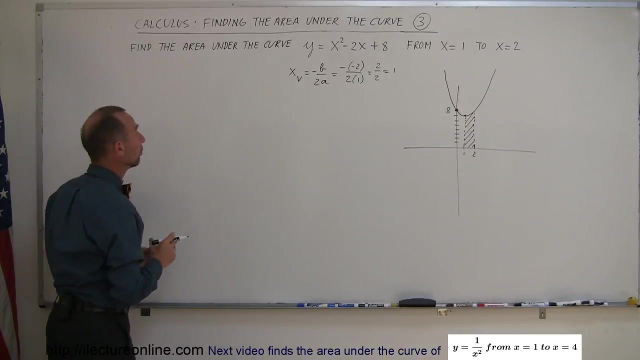 So it's fairly easy to grab a parabola even if there are no roots. Now we're supposed to find the area underneath the curve of this function: from x equals 1 to x equals 2.. So let's draw a line from x equals 1 down, And then here's the point 2.. Let's draw another line down here. So we're looking for the area underneath the curve. like that. It always helps to be able to have a visual picture of what we're trying to do. Okay, So now let's go ahead. The area underneath the curve is equal to the integral from x equals 1 to x equals 2.. 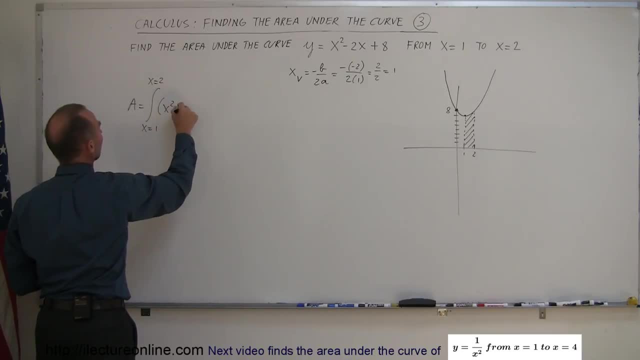 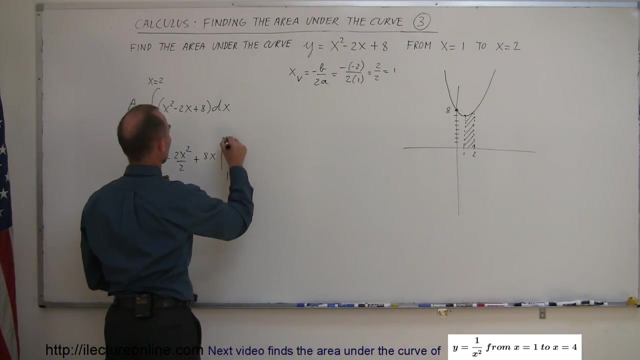 x equals 2 of the function, which is x squared minus 2x plus 8 times the dx, And that is fairly easy to integrate. So this is equal to x cubed over 3 minus 2x, squared over 2 plus 8x, And evaluate it from 1 to 2.. Alright, Let's simplify this a little bit. So the 2 is there. Cancel out. 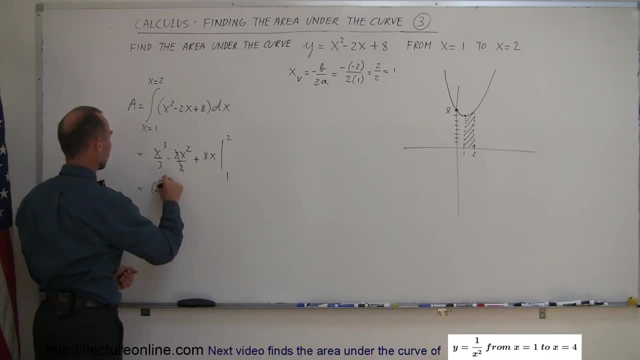 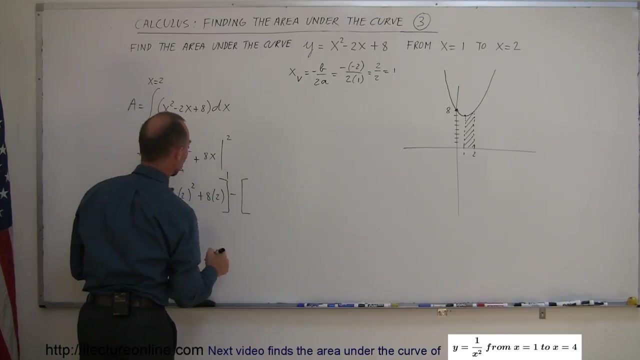 Now we plug in the upper limit, So we get this is equal to 2 cubed over 3, minus 2 squared, plus 8 times 2.. Let's put brackets around it. So this is what we get when we plug in the upper limit. Then we subtract from that when we plug in the lower limit, So plug in the lower limit, We get 1 cubed over 3 minus 1 squared and plus 8 times 1.. 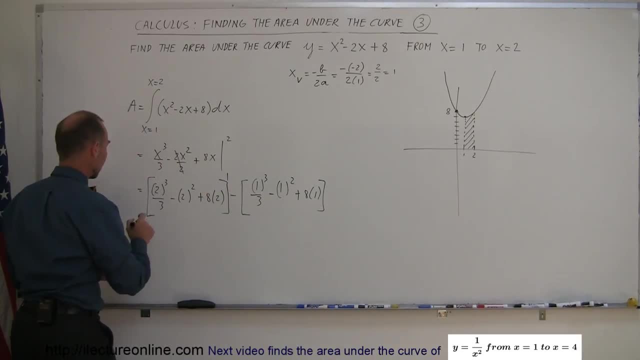 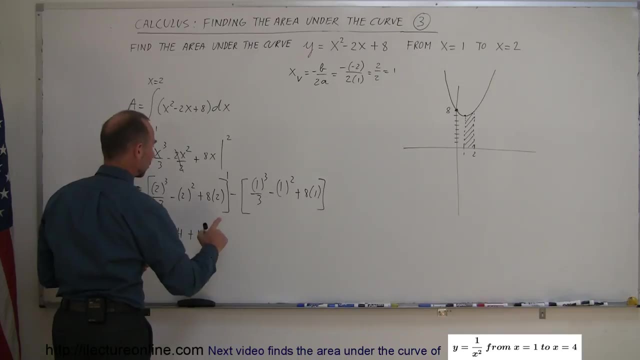 Okay, And working that out, we should get the measurement, the area. so let's see here: this gives us 8 over 3, minus 4 plus 16, and then we subtract from that minus 1 third. minus times a minus gives you a plus 1, and minus times a plus. 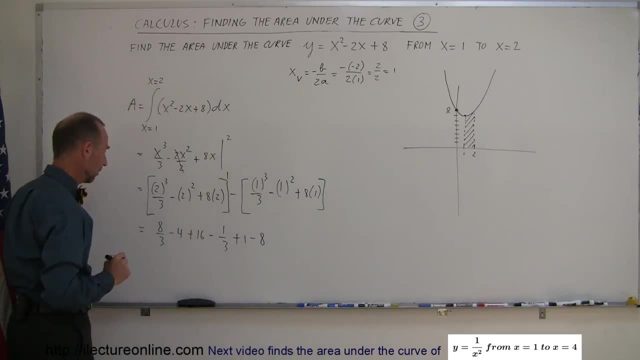 gives you minus minus 8.. All right, let's see if we can simplify this a little bit. We have 8 thirds minus 1 third, that's 7 thirds. We have a minus 4 plus 16, that's. 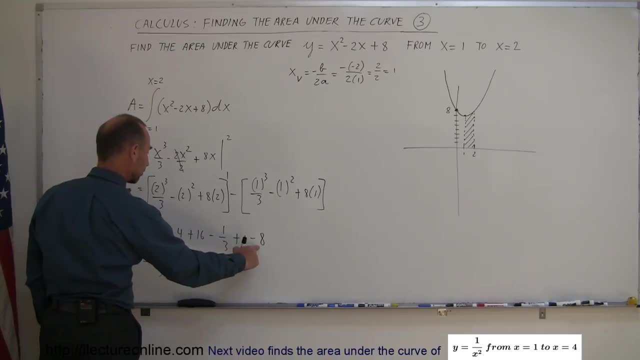 plus 12, minus 8, that gives us plus 4, plus 1 is plus 5, so that's plus 5, and 7 thirds is the same as 2 and 1 third, so it's equal to 2 and 1 third plus 5, so finally we can.